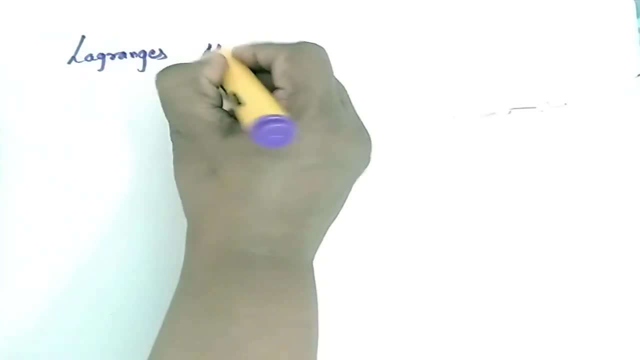 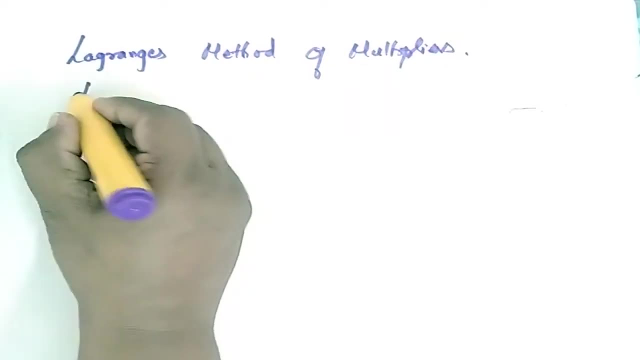 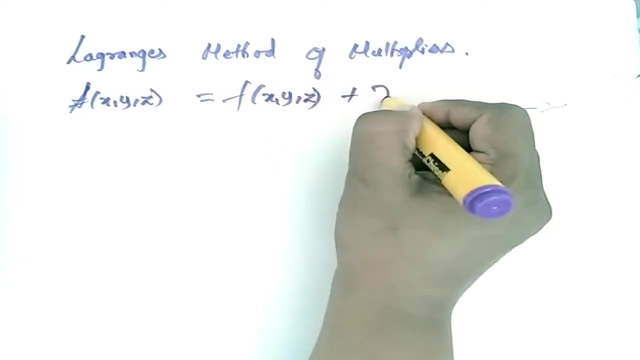 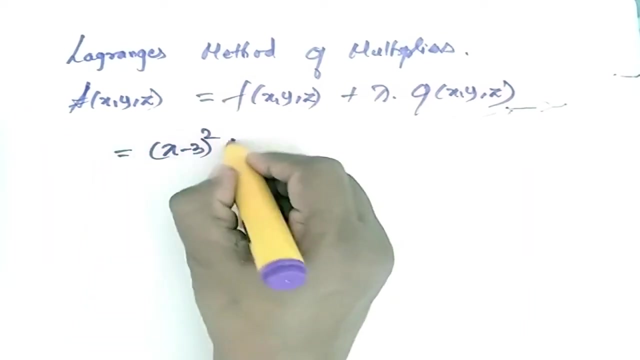 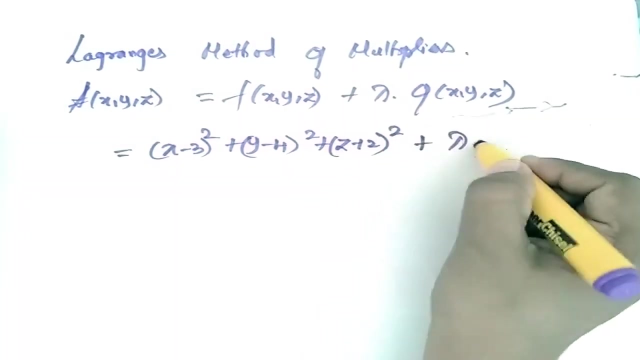 Lagrange's method of multipliers: F of x comma y comma z is equal to f of x comma y comma z, plus lambda into pi of x comma y comma z. So this is equal to x minus 3, the whole square plus y minus 4, the whole square plus z minus 12, the whole square plus lambda into x square plus y square plus z square minus. 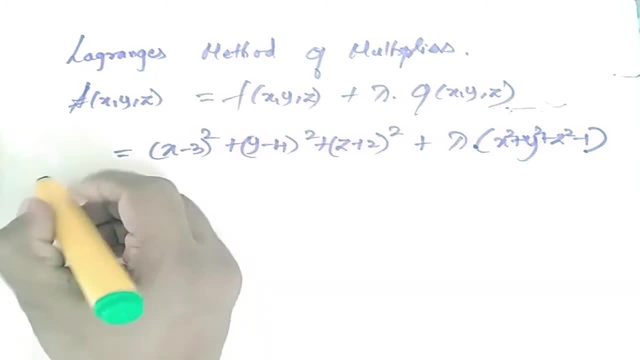 1. Now find dou f by dou x, dou f by dou y, dou f by dou z: 1. Dou f by dou x is equal to 2 into x minus 3 plus 2 lambda x. Dou f by dou y is equal to 2 into y minus 4 plus 2 lambda y. 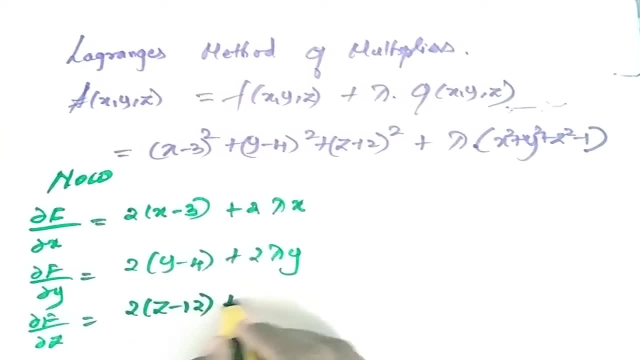 Dou f by dou z is equal to 2 into z minus 12 plus 2 lambda z. Now this is equal to 0.. This is equal to 0.. This is equal to 0.. So this implies lambda is equal to minus of x minus 3 by 3.. 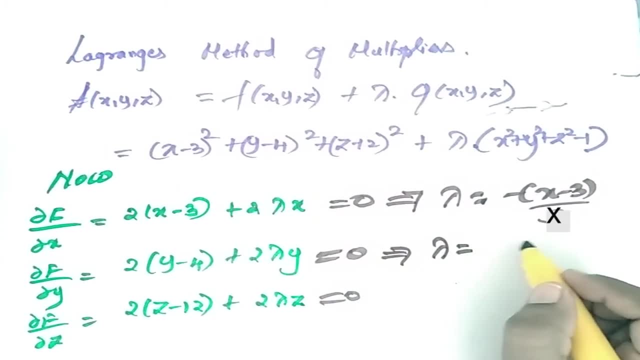 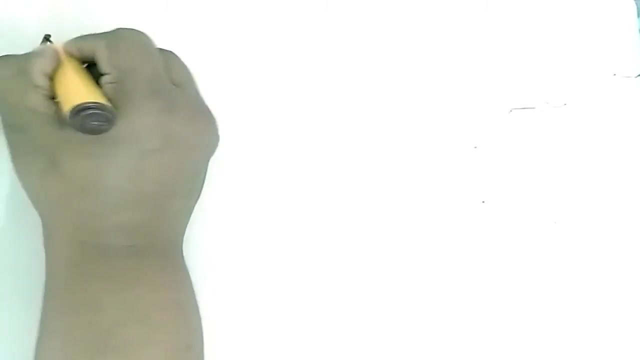 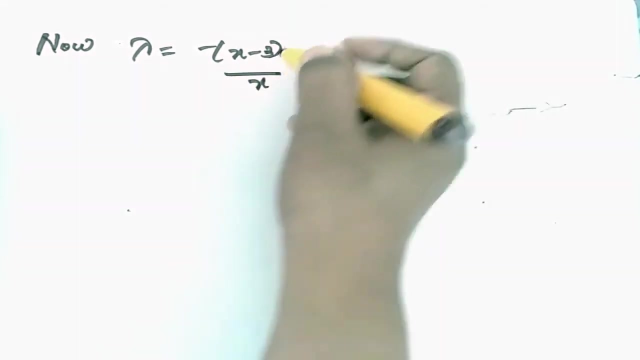 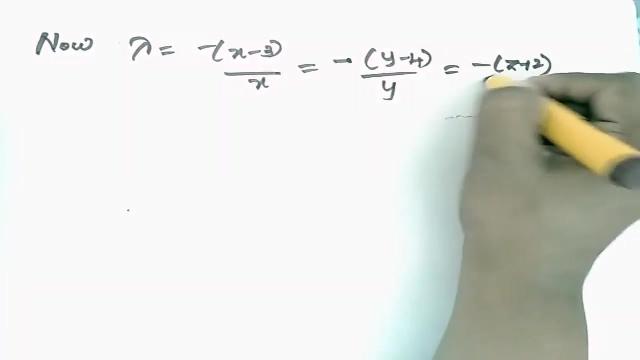 This implies lambda is equal to minus of y. This implies lambda is equal to z minus 12, minus of z minus 12 by z. Now, lambda is equal to minus of x minus 3 by x is equal to minus of y minus 4 by y, which is equal to minus of z minus 12 by z. 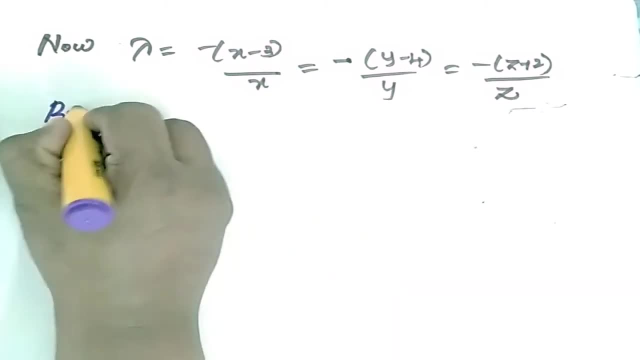 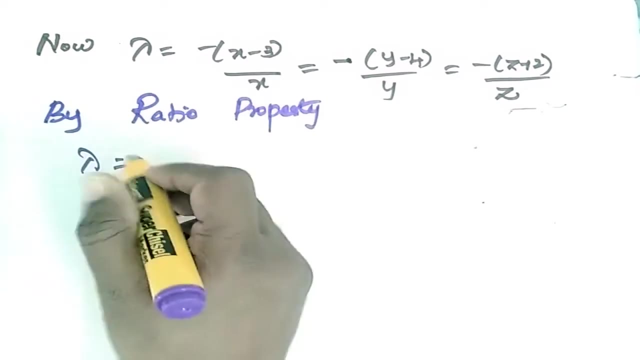 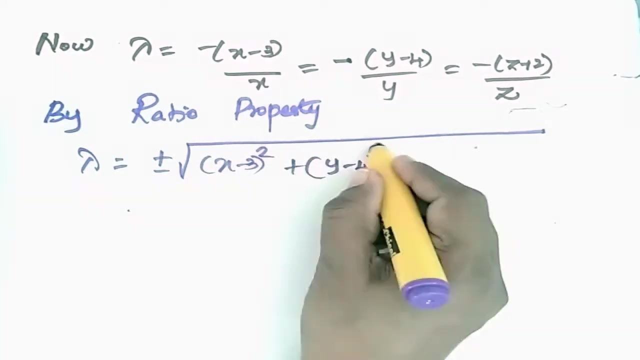 By ratio. By ratio, property Lambda is equal to plus or minus square root of x minus 3, the whole square plus y minus 4, the whole square plus z minus 12, the whole square by square root of x square plus y square plus z square. 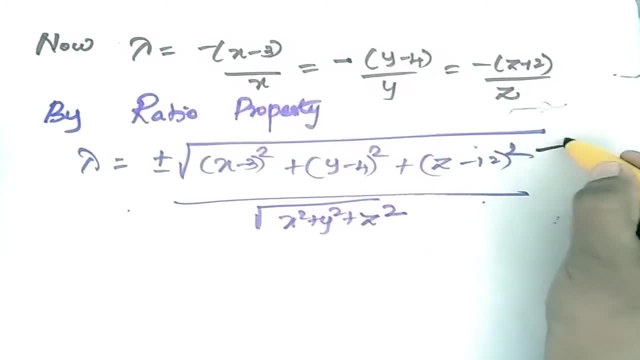 So now this is equal to Square root of f of x comma. y comma is z. So lambda is equal to plus or minus square root of f by this is equal to 1.. So this is 1.. So this implies lambda is equal to plus or minus root f. 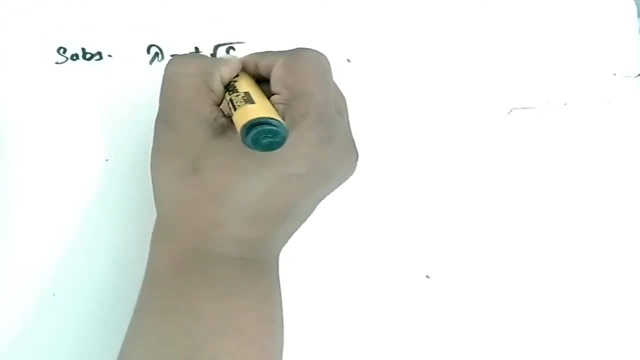 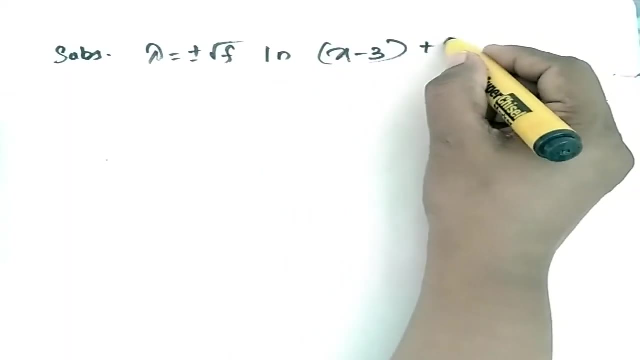 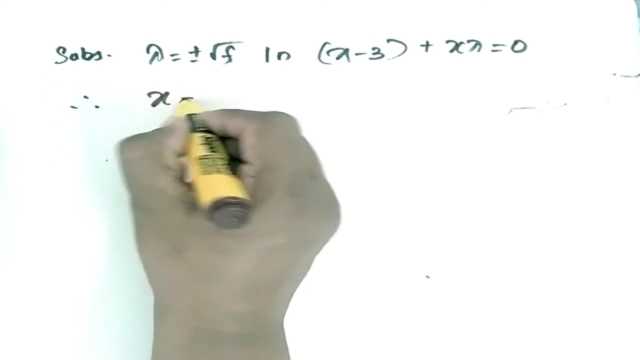 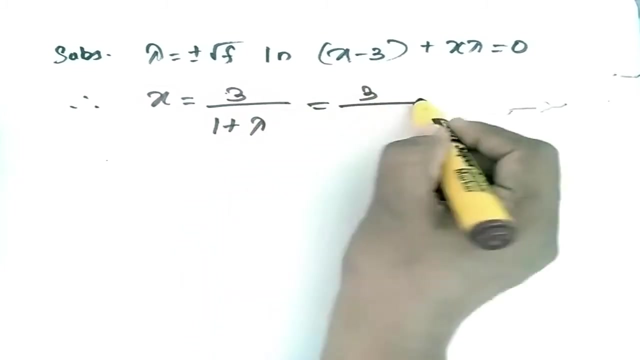 Substitute Lambda is equal to plus or minus root f. in x minus 3 plus X, lambda is equal to 0.. So therefore, x is equal to 3 by 1 plus lambda, which is equal to 3 by 1 plus root f. 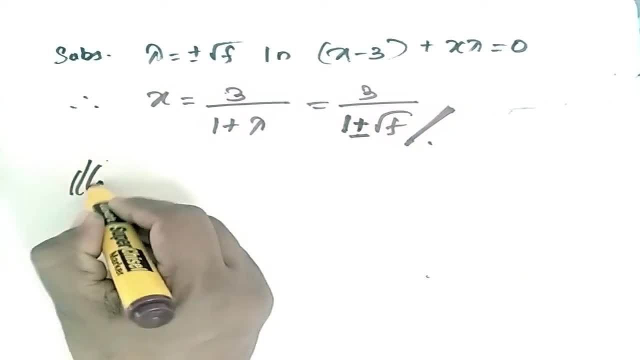 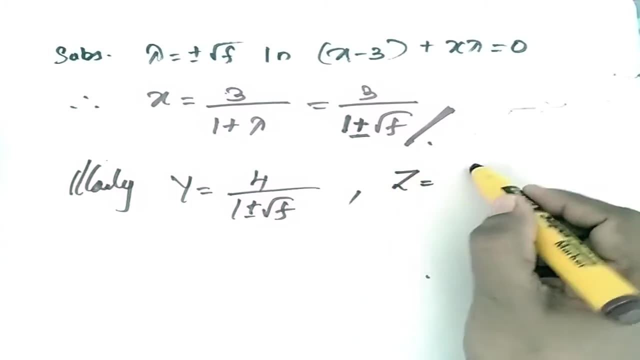 So minus root f. Similarly, y is equal to 4 by 1 plus or minus root f. Z is equal to 12 by 1 plus or minus root f. X square plus y square plus z square is equal to 1.. 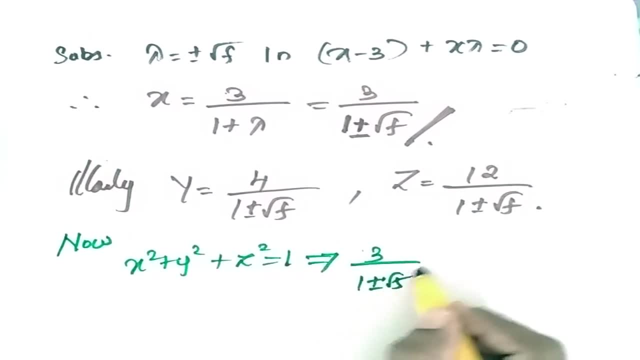 Implies 3 by 1 plus or minus root f, the whole square, plus 4 by 1 plus or minus root f, the whole square. plus 12 by 1 plus or minus root f, the whole square is equal to 1.. So this implies: 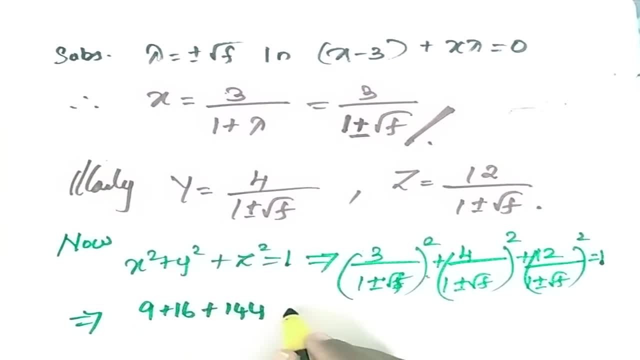 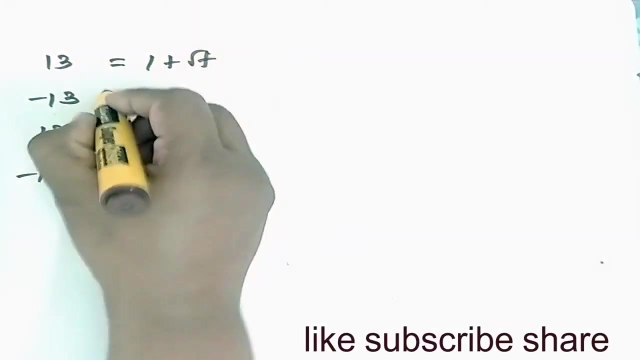 9 plus 16 plus 144 is equal to 1 plus or minus root f, the whole square, So this is equal to 169. is equal to 1 plus or minus root f, the whole square. So this implies 13 is equal to 1 plus or minus root f, 13 minus 13,. 13 minus 13 is equal to 1 plus root f. 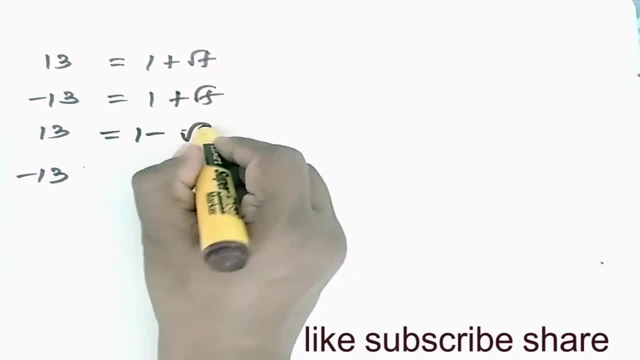 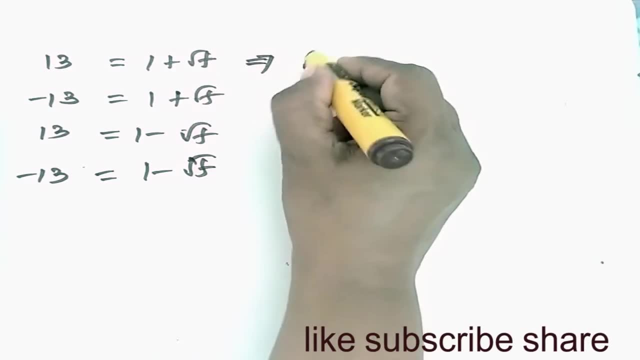 1 plus root f, 1 minus root f and 1 minus root f. So these are all the possibilities. So from this, root f is equal to 12, root f is equal to minus 14, root f is equal to minus 12, root f is equal to 14.. So these two values are not possible.